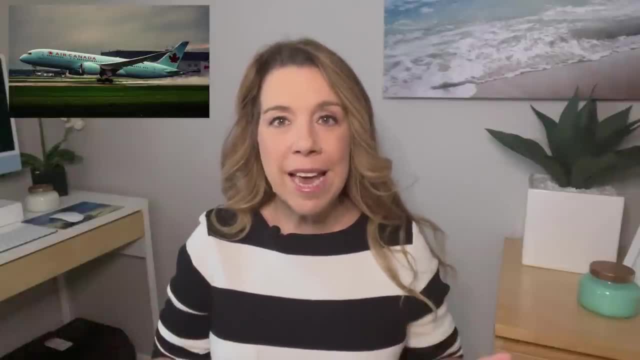 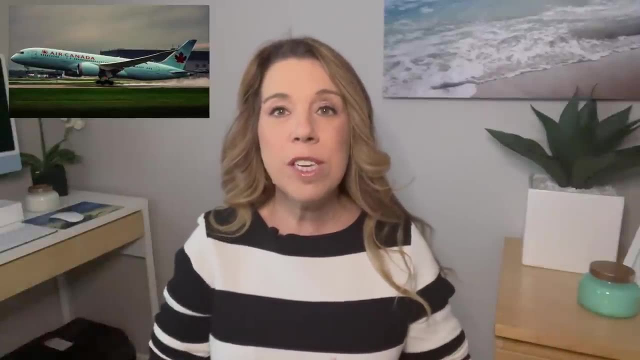 the advice that we always hear: fly in one day before your cruise. Yes, and typically I do say fly in one day before your cruise, but when you are going from North America, in particular, and you're going to Europe, you want to do two days before your cruise. at a minimum you could. 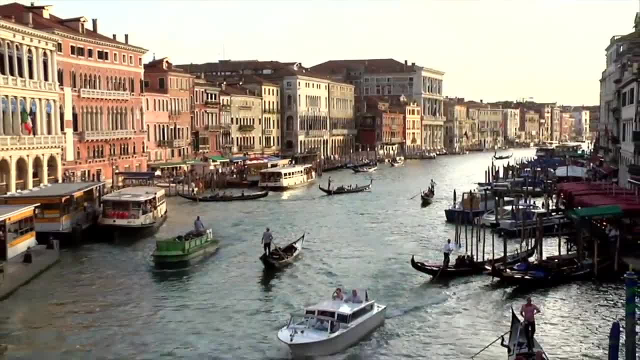 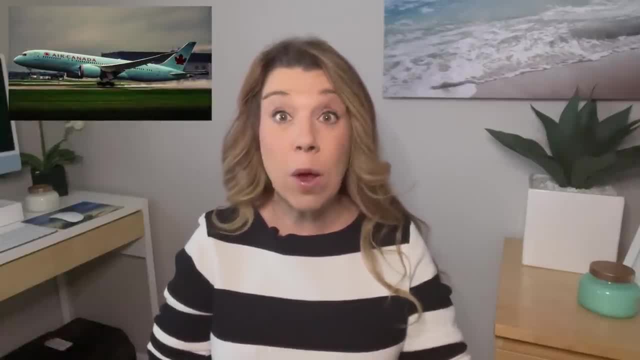 even do three days because, let's face it, you want to explore more, you want to visit that destination port a little bit longer. but by flying in just one day before we found, first of all, we were exhausted. there is the time difference, there's the jet lag, we were also 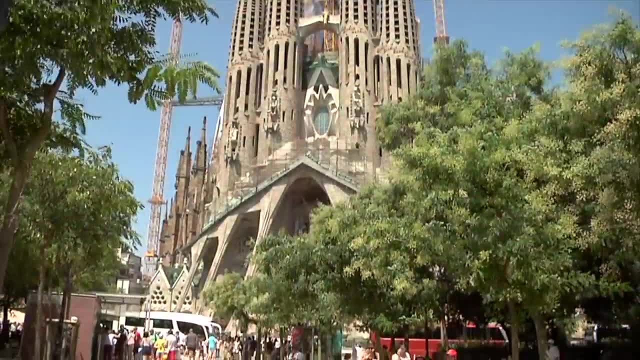 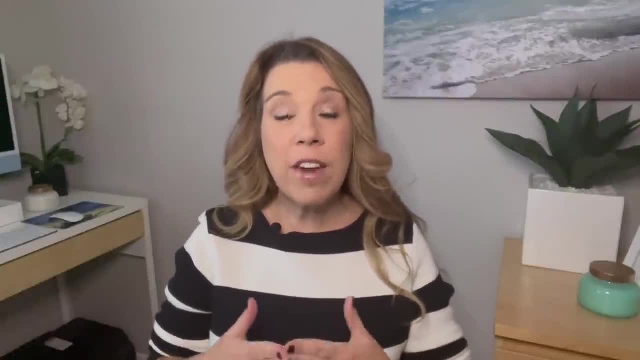 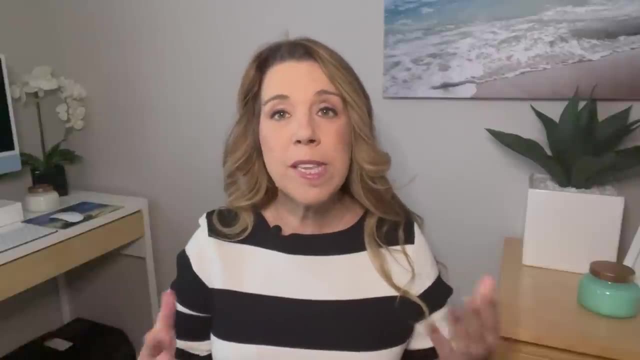 reclimated to a completely new city. we came into Barcelona- amazing city- and we were generally so, so tired and so so off on that very first day that we did arrive to Barcelona after our flight. so by the time we did start our cruise the next day, at least the good thing was we weren't tired. 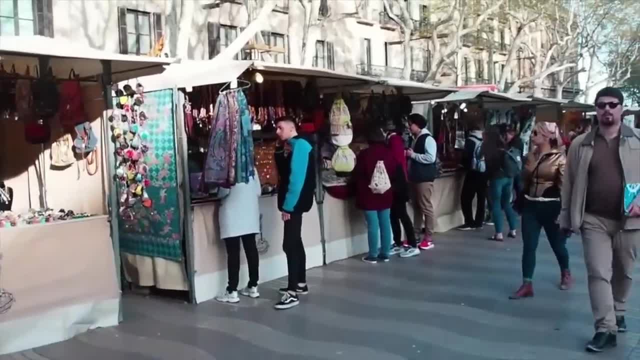 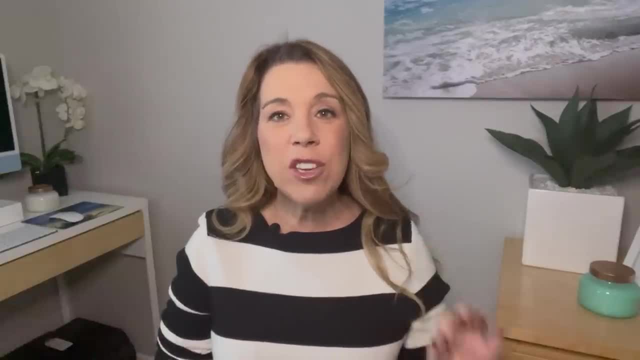 for our cruise, but had we arrived two days before, we would have really had more time to explore Barcelona, be less tired and really I think it is good advice to do that. Take two days before your cruise, especially if you're going on a Mediterranean cruise for the 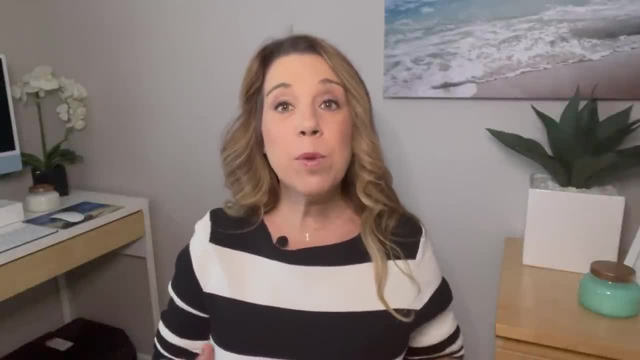 first time. Number two: we made the mistake of thinking that, because we were visiting pretty popular tourist destinations, that everybody would speak English and we would really have no need to learn a little bit of the local languages. and I just think, when I look back I think, well, that was. 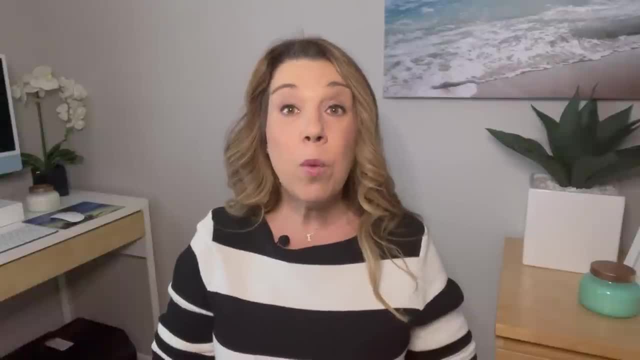 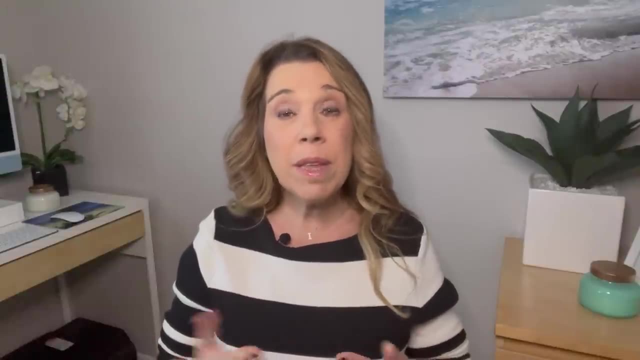 really kind of naive, maybe a little bit ignorant, on my part. what I really should have done is learned at least a few common phrases for each of the different destinations that we were at, something that you can do as well as you can download an app. I'll see if I can find a good one. 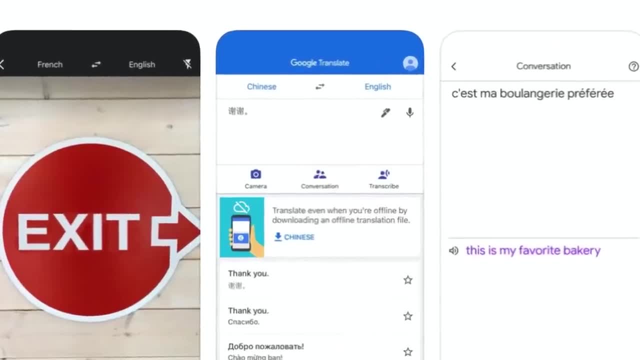 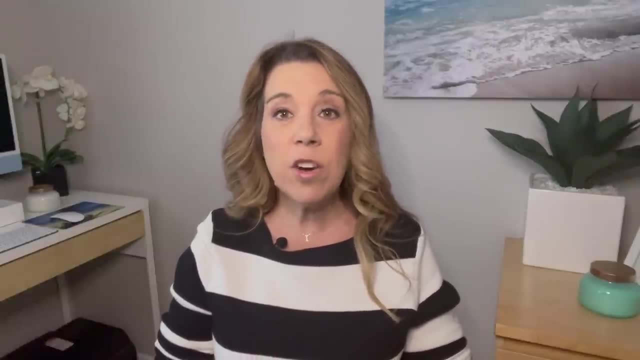 and I'll leave it on. I'll screenshot it on the screen. I think it really is helpful, and something that we did notice is, while we were always able to be understood, like in a taxi cab or even in a restaurant, if we did go a few streets away from any of the main part of the tourist area in any 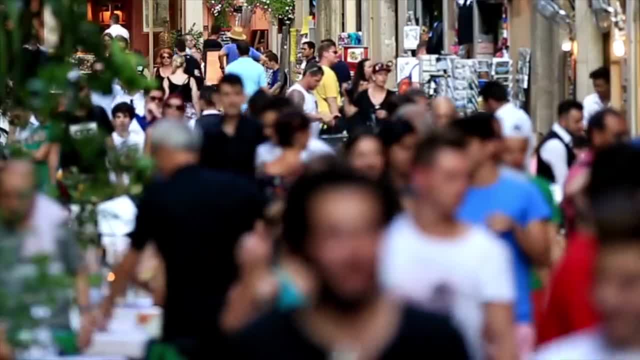 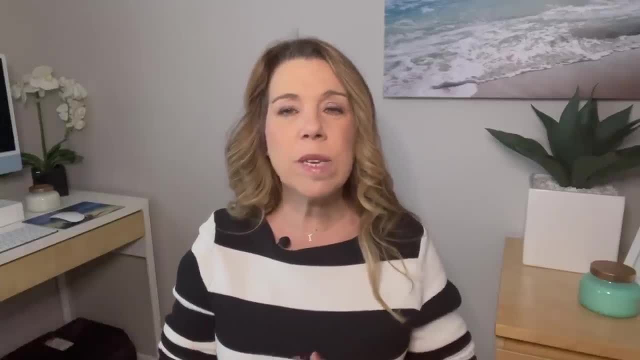 of the different cities that we went to. even in some place like Rome, for instance, just by going around the city we were able to speak as much English as we thought, and I just think it goes a little bit of a way to show a little bit of respect to the local population, to the local. 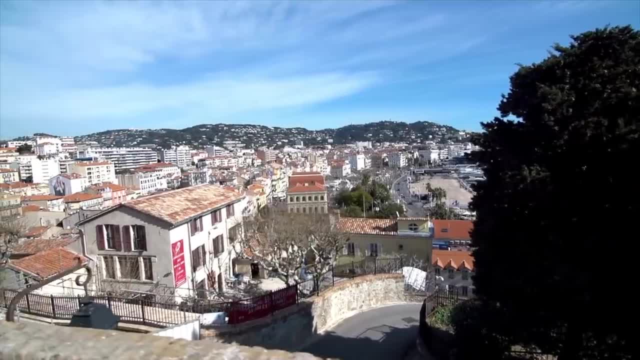 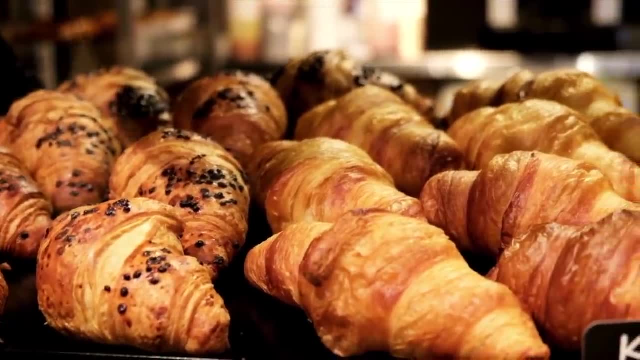 people when you do speak or try to speak a little bit of their language. Now, we definitely noticed this because when we were in France, we went into a boulangerie and we ordered some croissants, and I think it was a pastry called the Saint Pierre. anyway, it's so good and we speak French as a 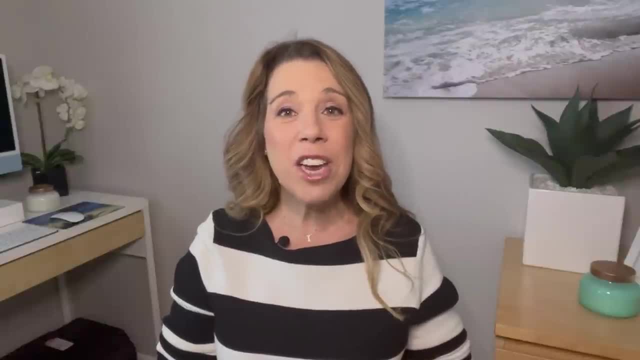 second language and we were able to speak with the people who worked in the shops in French and you know, and they really, really interacted with us. it was really, really pleasant. so I do think if you could learn a little bit of the language or at least get a few common phrases, it does go a long. 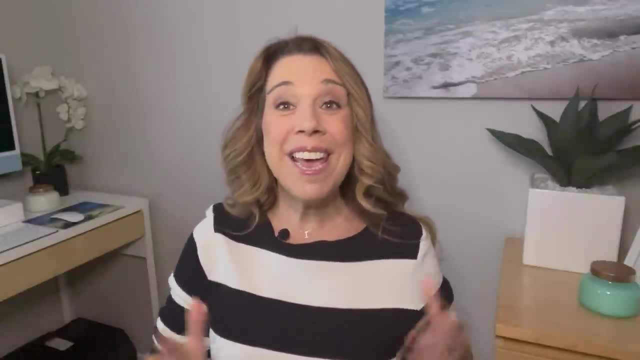 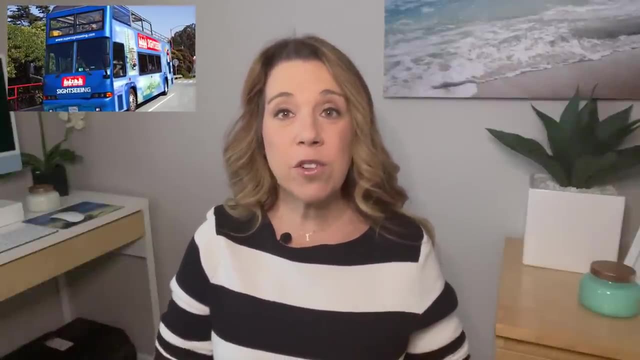 way. Number three: not taking advantage of the hop-on, hop-off buses in many of the different destinations that we were in. now, what we did before our cruise is: we mostly booked all cruise line excursions with the exception of one. we did a private excursion in Ephesus and Koussidasie. that 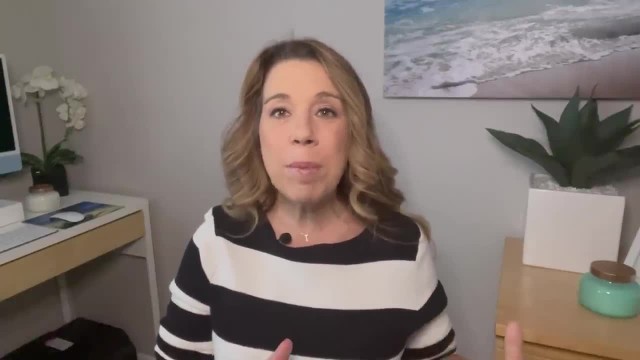 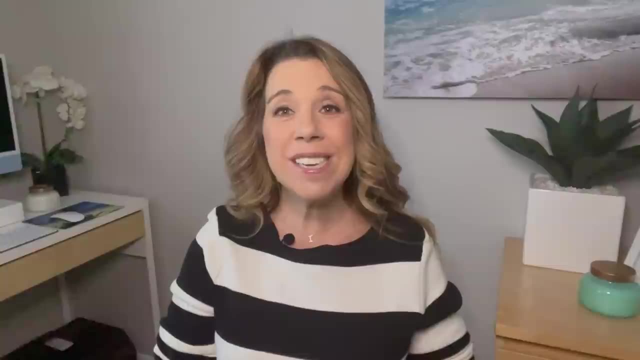 was only half a day. I had really researched this quite well and I did know somebody who had taken taken this tour with this company and it had gone really well. so we did book that one privately- a very good decision. the rest of them we really booked with the cruise line and while this was, 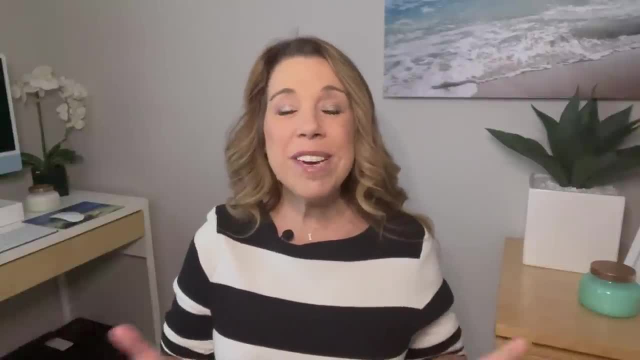 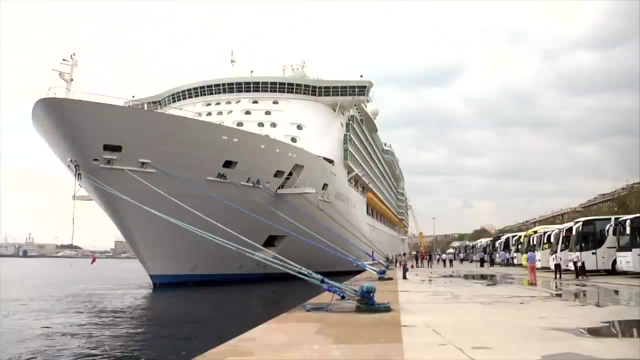 a good decision in terms of getting back to the ship on time. there were definitely some ports that we could have explored with the hop on, hop off buses. we could have just timed our day to make sure that we did get back to the cruise port on time. but not only would this have saved money, but 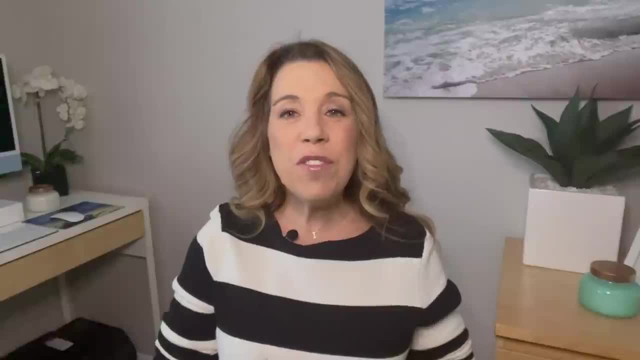 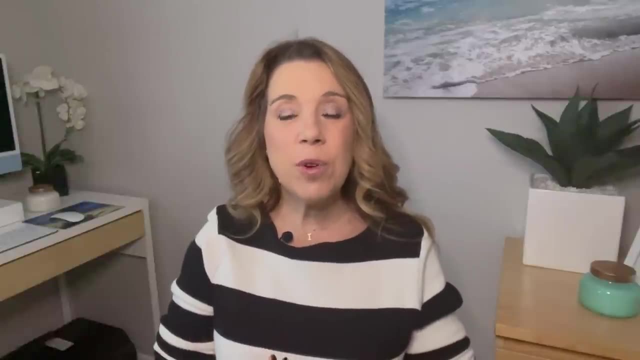 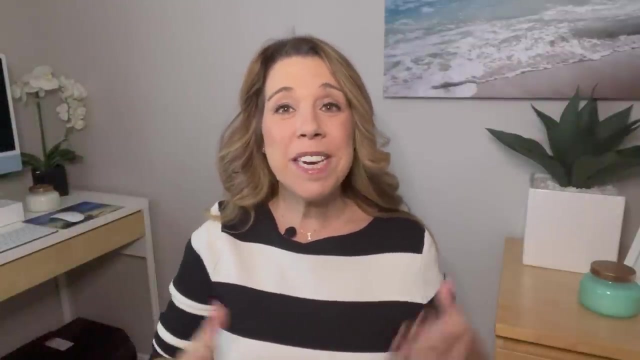 more importantly, we wouldn't have been maybe grouped with 50 to 100 other people, which in some cases we did find that it was hard to hear the guide during our excursions and we kind of regretted not researching this a little bit more. number four: expecting that the shops and even the 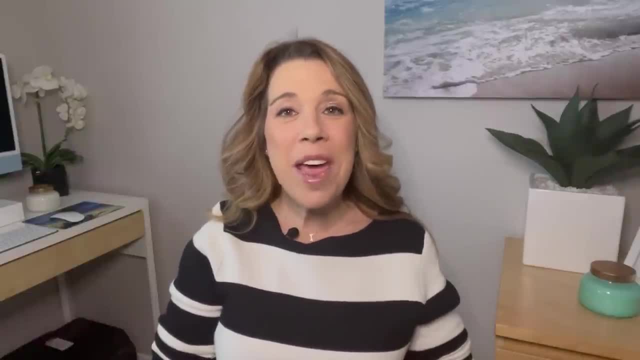 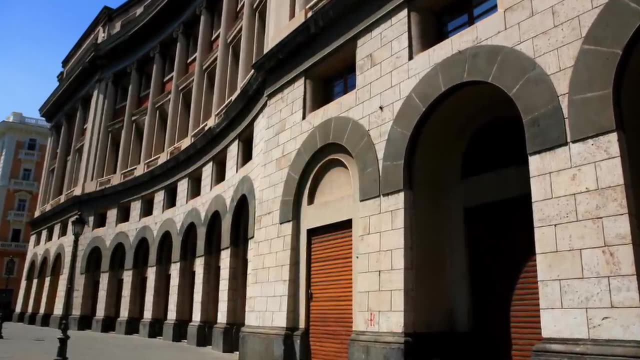 restaurants would be open all day now. what i mean is when we went into some of the different towns. well, these shops did close down, oftentimes between like 1, 30 and 2 o'clock, and then they closed down and we were able to get back to the ship on time. and we did get back to 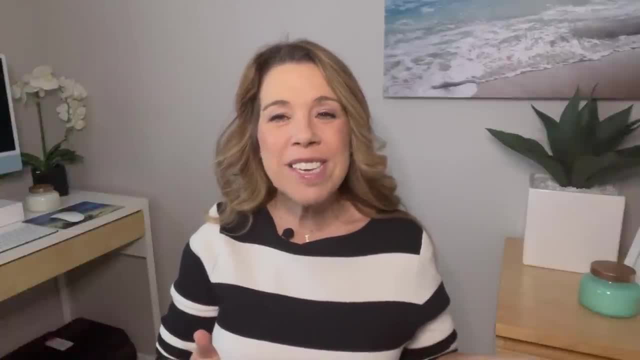 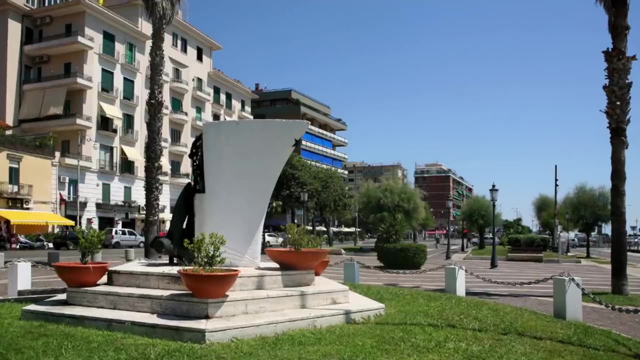 the ship on time and four o'clock in the afternoon now. while i had heard about this ahead of time, i just didn't think this would be in the actual cruise ports, but this really did happen. we were walking in salerno in italy in the afternoon that we had done a pompey excursion in the morning time. 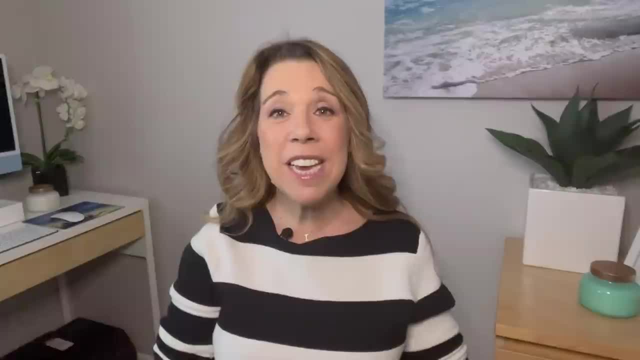 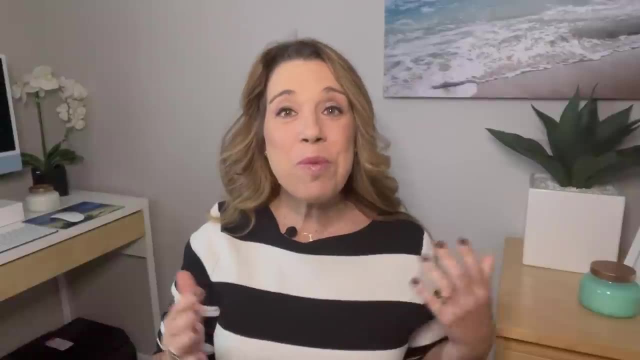 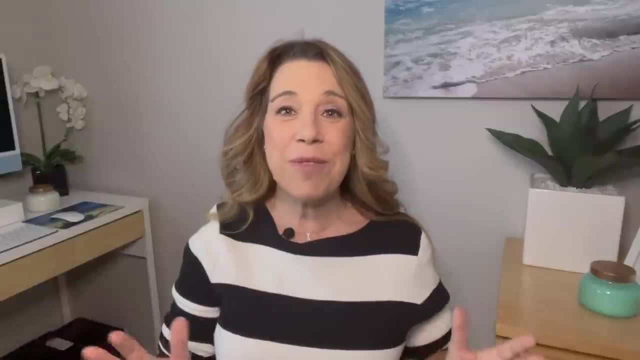 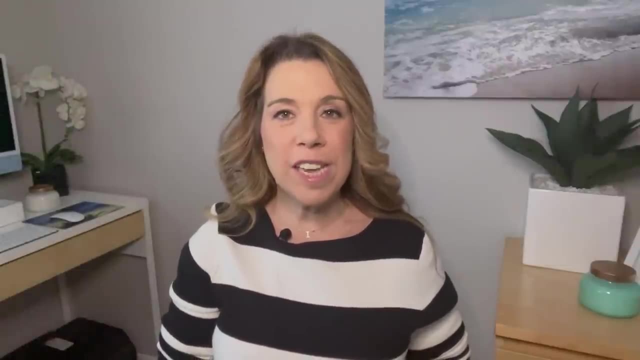 to like the united states and customer service. it really is different when you are in a lot of those mediterranean cruise ports. number five: choosing the early dining or the early seating. now, this was definitely a mistake for us, given our cruise ports and the fact that many times we had excursions that were between like eight and ten hours for the day, so we would get back on the cruise ship maybe at five or even sometimes close to six, and our dinner time, i believe in the mediterranean it was at 6: 30 pm, so we were really rushing to go to dinner. and oftentimes we weren't even really that hungry at that time. so it would have been better in hindsight that we had booked maybe the late dining at maybe 8: 30 pm or 8 o'clock pm and in the case of open dining, which is available on so many cruise ships now, i think even booking something. 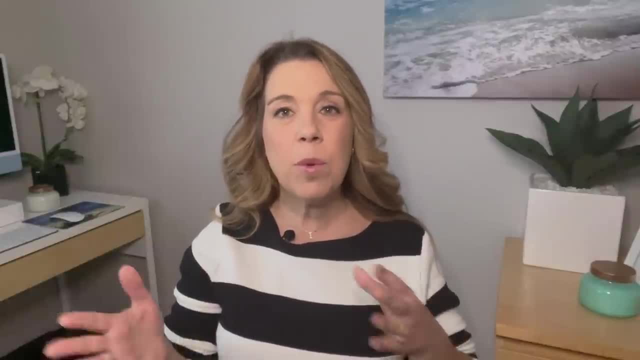 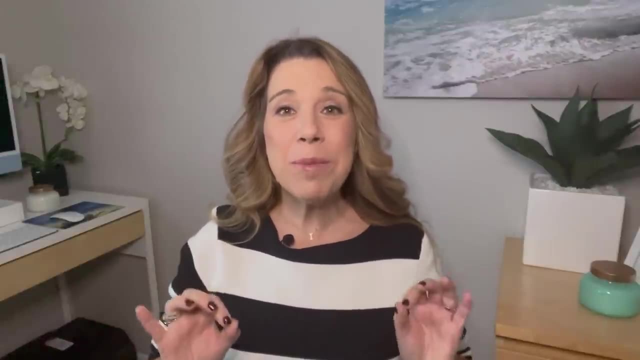 that's after 7, 30 or 8 pm, obviously, depending on you and when you like to eat. but this really would have been something that would have been better for us. now i am going to tell you the one thing that we did really, really right in just a minute. but first this is number six. this is kind 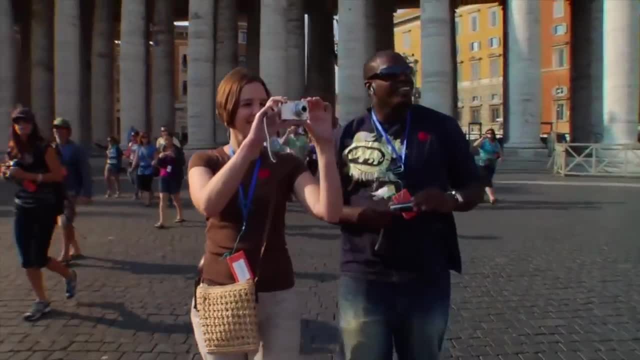 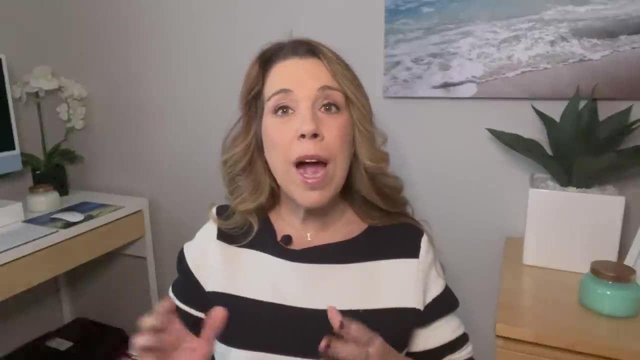 of tip. be very careful when you are booking cruise line excursions, when you look at the description of it. if you see things like a turkish rug demonstration. if you see other things like a perfume factory tour, if that's part of the excursion, sometimes you are spending a lot of. 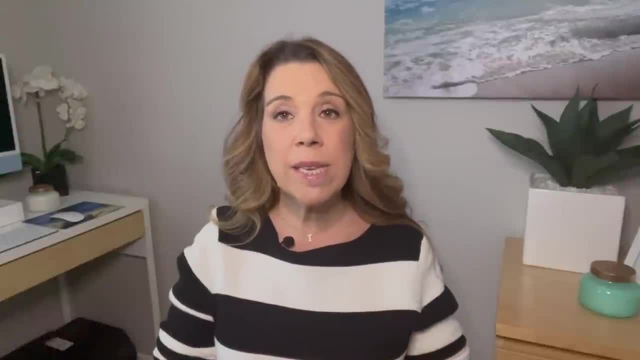 time in those places, in that demonstration, let's say, and while it starts off as being a little bit interesting, after about 45 minutes it turns into a sales pitch. and what we found is when we had a shore excursion that was, let's say, four to maybe five. 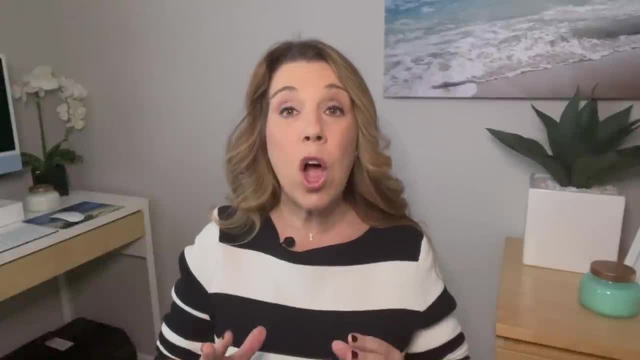 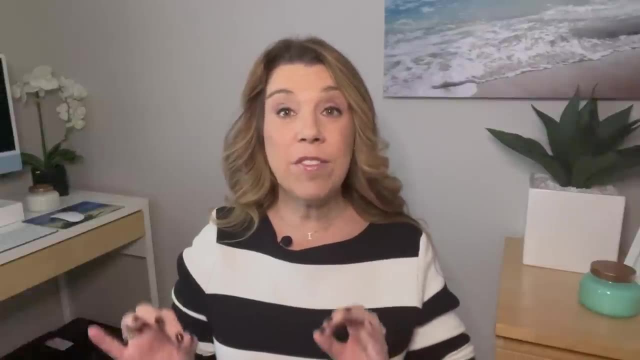 hours, that we maybe spent an hour and a half or longer in that demonstration or in that tour, and it's definitely something that if we could do again, i would definitely avoid any of those type of excursions. now, if you're not sure about it, you can actually speak to the people who work on the